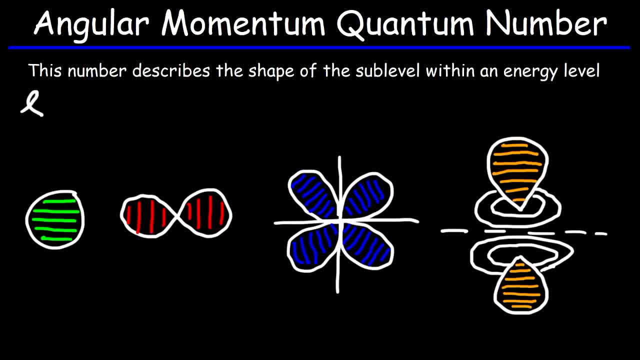 within an energy level. Now we have four energy levels. There are four different sub-levels that you're going to see on a regular basis. The first one is the S sub-level, which is basically a sphere. The second one is the P sub-level, and then we have 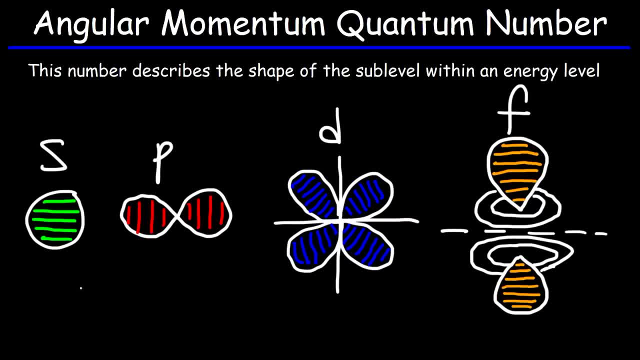 the D sub-level and the F sub-level. Now what you need to know is that for the S sub-level, L is always 0.. For P, L is 1.. For D, the angular momentum quantum number is 2.. And for F. 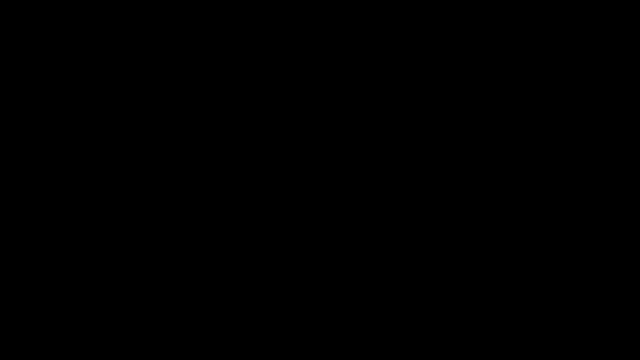 L is always 3.. Now let's talk about the relationship between N and L. L is less than or equal to N minus 1, and L and N are both integers, So let's talk about what this means. When N is 1, L can. 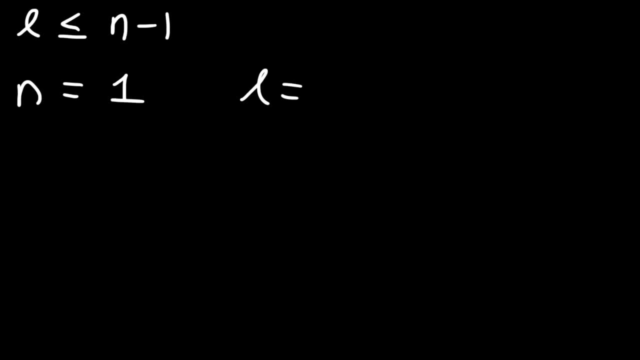 only have one value, That's N minus 1 or 1 minus 1, which is 0.. Now, when N is 2,, according to this equation here, L has to be less than or equal to n minus 1, or 2 minus 1,, which is 1.. 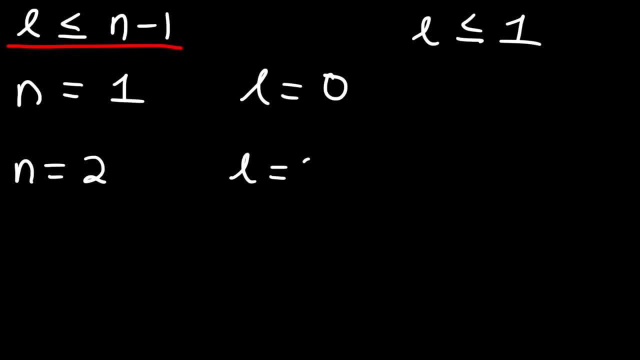 So that means L could be 0 or 1.. And this expression will be true. Now, what about when n is 3?? When n is 3, the maximum that L can be is 3 minus 1 or 2.. So L can be 0,, 1, or 2.. 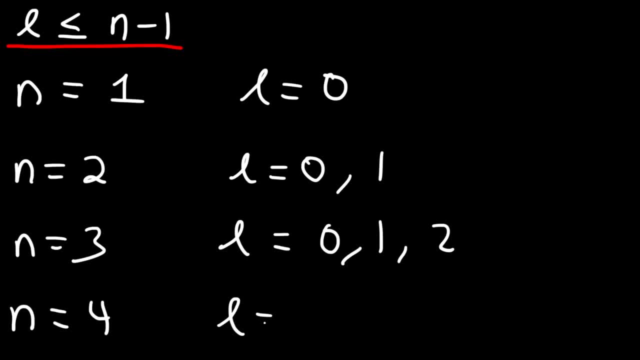 So when n is 4, L could be 0,, 1,, 2, or 3.. Now let's think about what this means. So remember, when L is 0, what sublevel do we have? When L is 0, this corresponds to S. 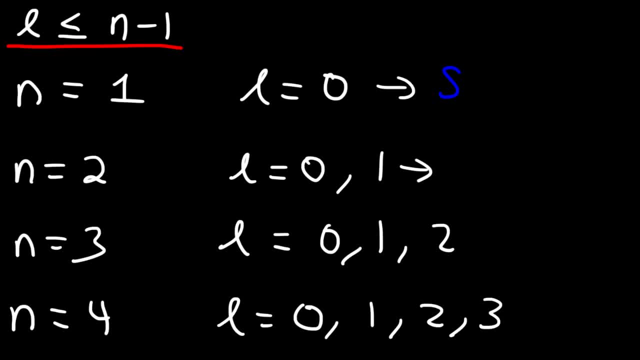 Now, when n is 2, L could be 0 or 1, which means that we can have the S or the P sublevel. When n is 3, L could be 2.. So we can have the S, P or D sublevel. 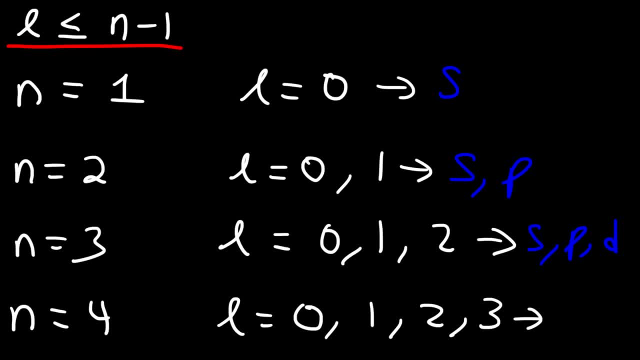 And when n is 4, we can have the S, P, D or F sublevels. Now notice that there's no 1P sublevel. This does not exist. The first energy level doesn't have the P sublevel. 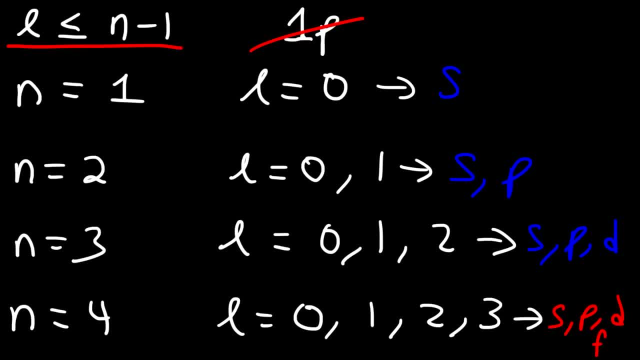 And let's say, if you were to write the electron configuration for an element, you'll know that there is no 2D sublevel. You have 2S and 2P, but not 2D. In the third level, you could have 3S, 3P, 3D, but not 3F. 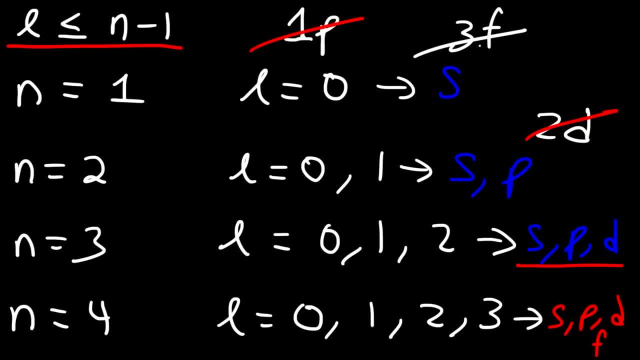 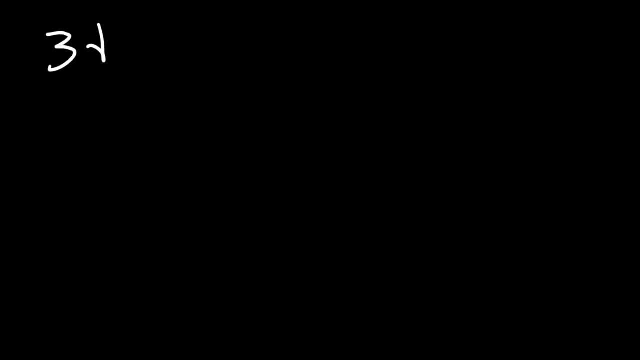 So 3F is not possible. Now you could have 4F. That's possible. Now here's a question for you. Let's say we have an electron in the 3D sublevel. Based on that information, what is the n value and the L value? 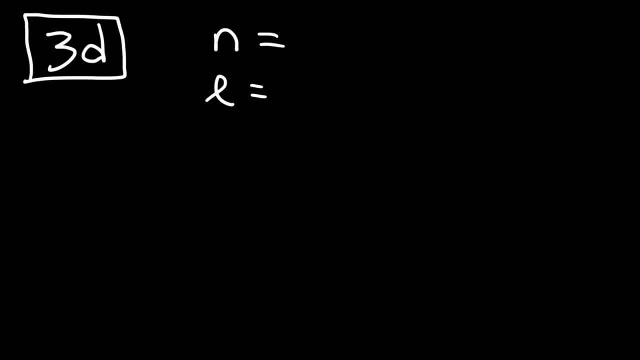 that corresponds to an electron in the 3D sublevel. n is basically the number that you see here. So n is 3.. Now for the D sublevel, L is what value? So, if you recall, for the S sublevel, L is always 0.. 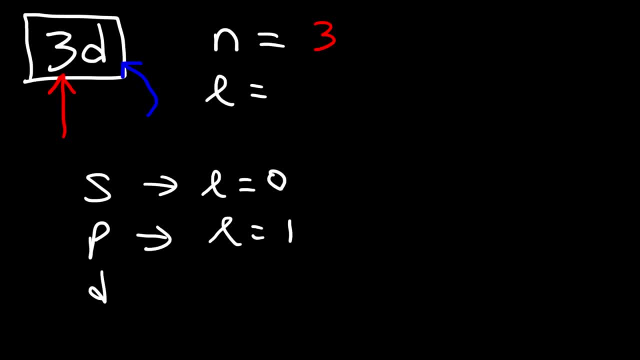 For the P sublevel, L is 1.. For the D sublevel, L is 2., And for the F sublevel, L is always 3.. So for the 3D sublevel, n is 3 and L is going to be 2.. 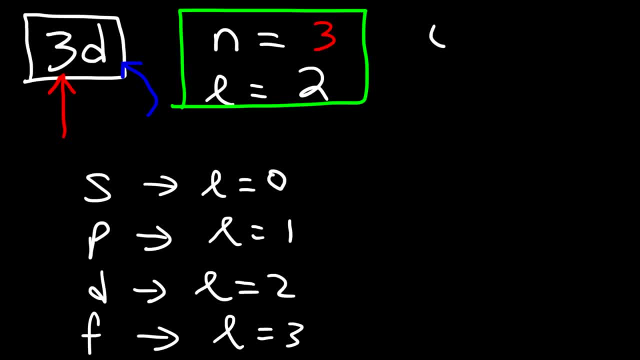 So let me give you another example. What if we have an electron in the 4F sublevel? What's n and what's L? As you can see, n is the number in front of F, so n is 4.. And F always corresponds to an L value of 3.. 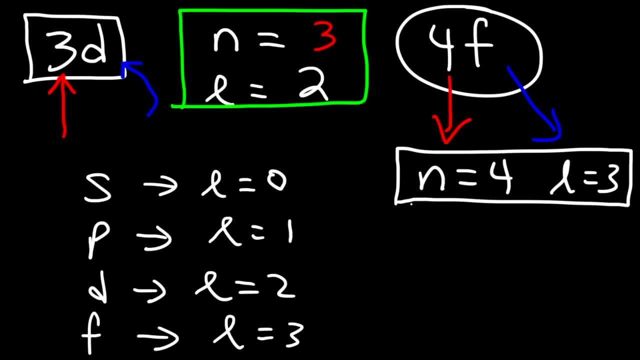 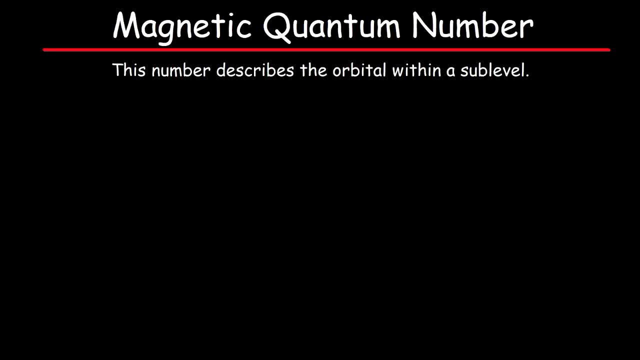 So for an electron in the 4D sublevel, n is 4F sublevel and it's 4LS3.. Now let's move on to the third quantum number, which is the magnetic quantum number, represented by the symbol m sub L. 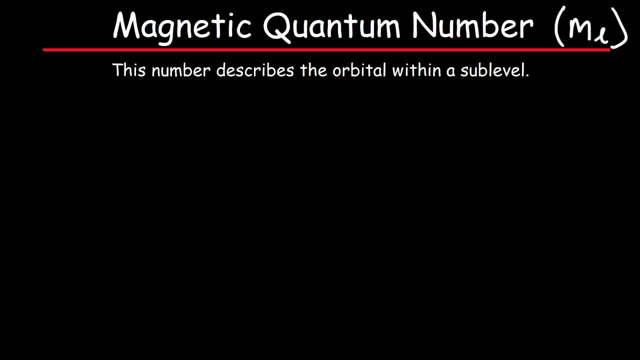 This number describes the orbital within a sublevel. An orbital is basically a region in space in which the probability of finding an electron is very high. In an orbital, an electron can have an upspin or a downspin, And so every orbital can hold a maximum of two electrons. 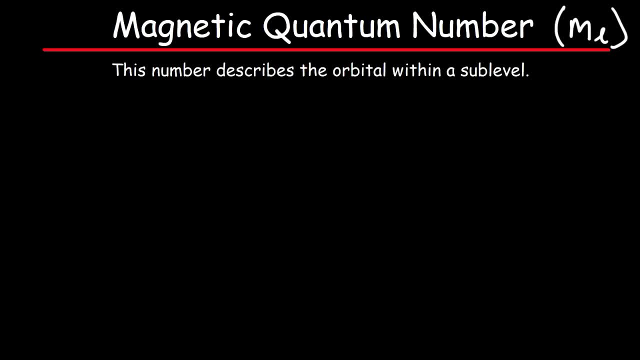 But now let's talk about the relationship between L and m sub L. So, as we said before, L is the angular momentum quantum number, m sub L is the magnetic quantum number. So when L is 0, we have the S sublevel. 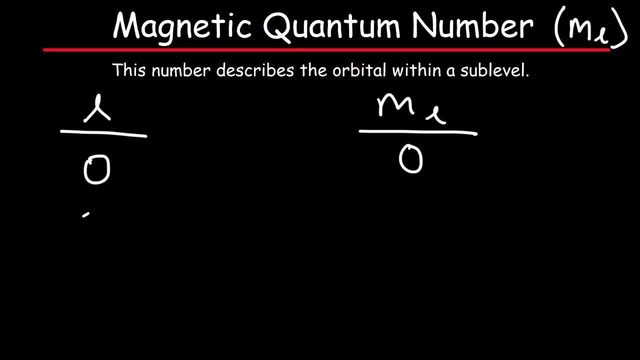 and mL can only be 0. When L is 1, we have the P sublevel and the P sublevel has a maximum of 2.. So we have the first sublevel and the second sublevel has a maximum of 1.. 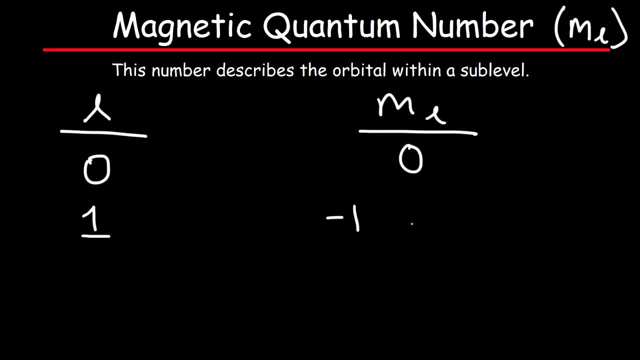 So when L is 1,, we have the S sublevel, and the P sublevel has a maximum of 2.. And so every orbital can hold a maximum of 2 electrons. three orbitals: The first one has the ML value negative 1,, the second one is 0, and 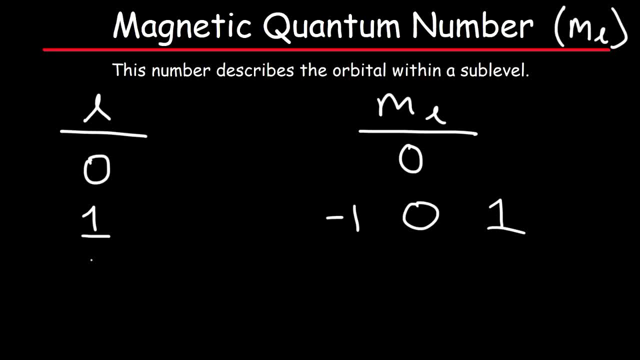 the third one has an ML value of 1.. When L is 2,, we have the D sublevel, and there are five D orbitals: negative 2, negative 1,, 0, 1, and 2.. When L is 3,, we have the F. 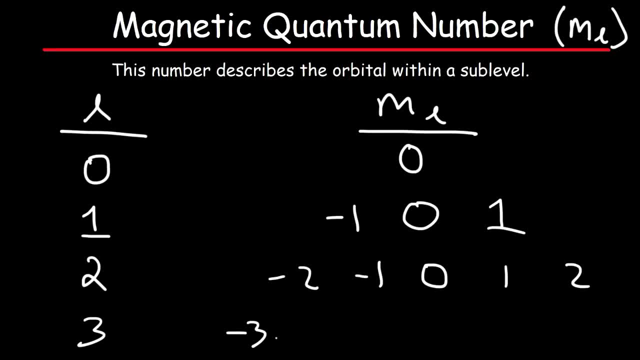 sublevel which has seven orbitals: negative 3, negative 2, negative 1,, 0,, 1,, 2, and 3.. So what you need to know is this ML is between negative L and L. So let's. 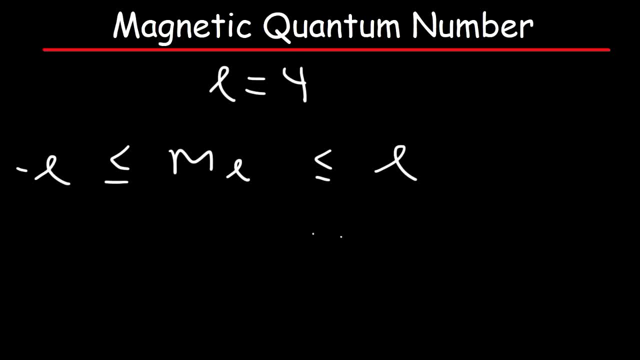 say, if L is 4, that means ML will be an integer between negative 4 and 4.. So it could be negative 4, negative 3, negative 2, negative 1, 0, 1,, 2, 3, 4.. So this: 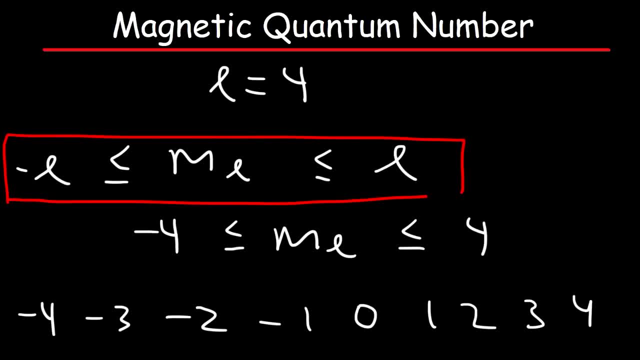 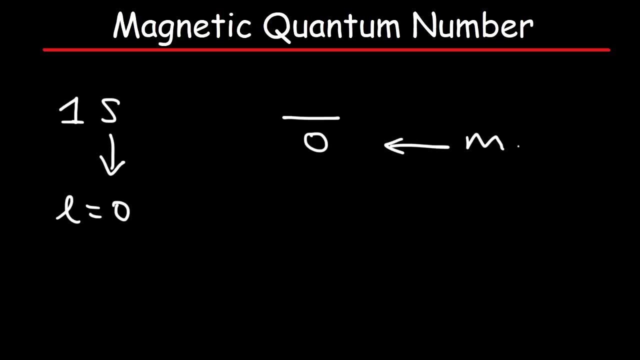 expression shows the relationship between ML and L. So let's say, if we have the 1s sublevel, S only has one orbital and for S, L is 0, and ML, which is this number, will also be 0.. Now let's say, if we're focused on the 2p sublevel, P has three orbitals. Now for 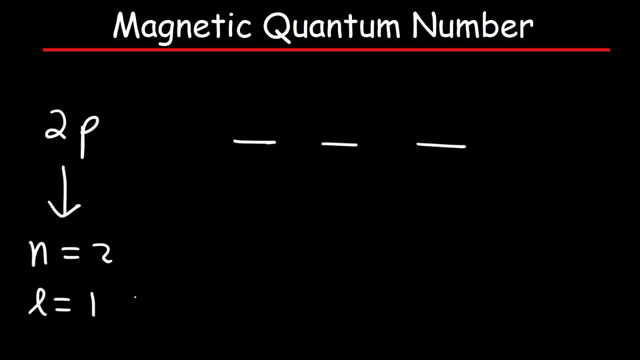 2p, we know that N is 2, and for P, L is always 1.. Because L is 1, ML could be negative: 1,, 0, or 1.. And so, as you can see, the ML values: they correspond to the specific orbitals within a sublevel. 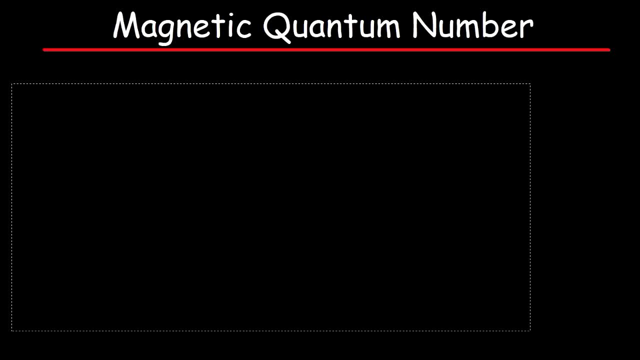 Now let's say if we have the 3d sublevel, where N is 3 and L is 2.. Now the d sublevel has five orbitals, which means that it can hold a maximum of 10 electrons, because you can put two electrons per orbital, Since L is 2, ML. 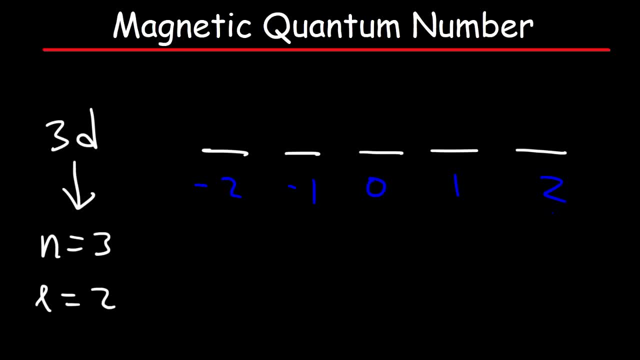 could be anywhere from negative 2 to 2.. And so each ML value corresponds to a specific orbital in the sublevel. Lastly, let's go over 4f, where N is 4 and L is 3.. The F sublevel has seven. 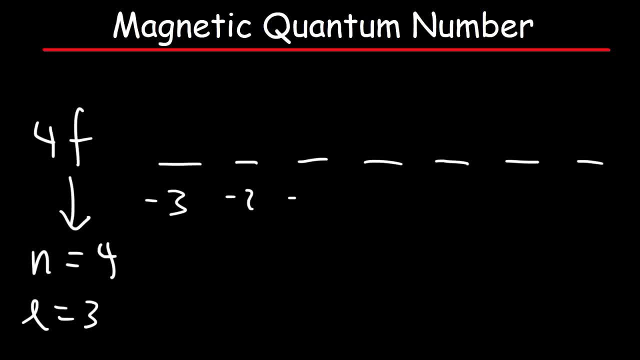 orbitals, Where ML can vary between negative 3 and positive 3.. So hopefully this helps you to see the relationship between L and ML, which gives you these numbers. Now, the last quantum number that we need to talk about is something known as the electron. 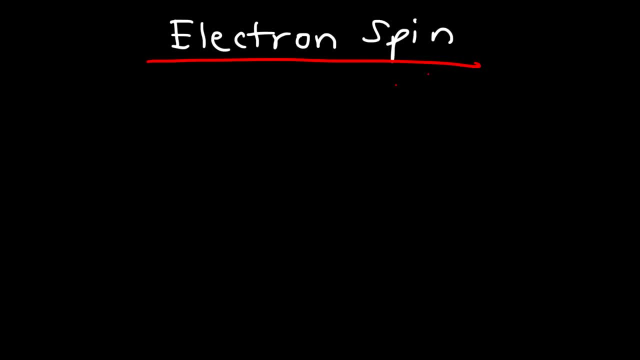 spin. The symbol that corresponds to this is m sub s. Now the electron spin could be one of two values: positive or negative. 1 half. Now recall that an electron within an orbital can either be going up or down. So if it's going up, 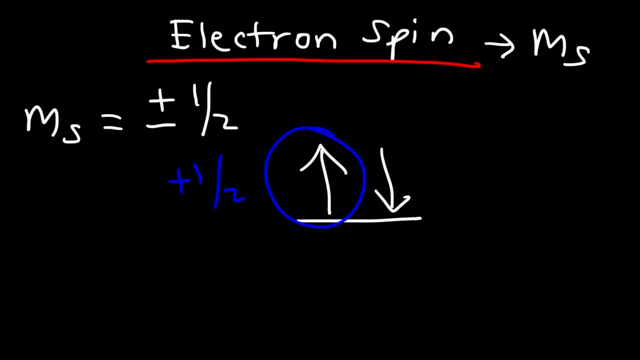 the spin is positive 1 half And if the arrow is going down, the electron spin is negative 1 half. So that's the last quantum number that you need to be familiar with. Now, let's say if we have the 3d 8-electron. 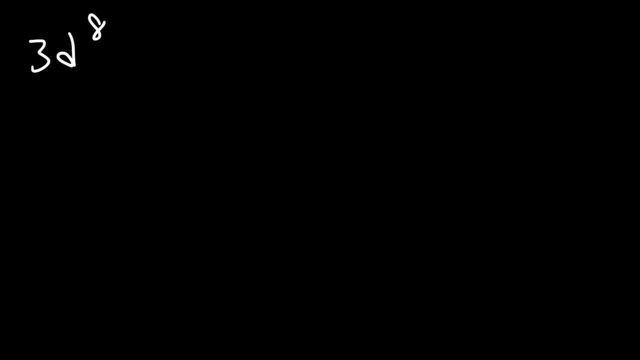 What are the four quantum numbers that correspond to the 3d 8-electron? What would you say? Well, we know that N has to be 3 based on this number, And for the D sublevel, L is always 2.. Now we know that D has five orbitals, And so the ML values will. 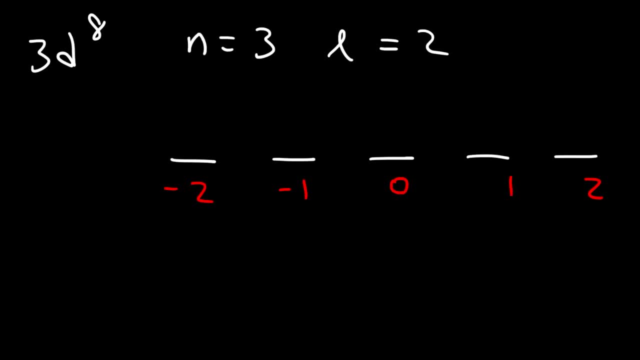 range from negative 2 to 2.. Now we need to find the location of the 8-electron. The location will tell us the ML value and also the ms value. Now, ms will always be either positive or negative 1 half, which I'll explain shortly. So let's 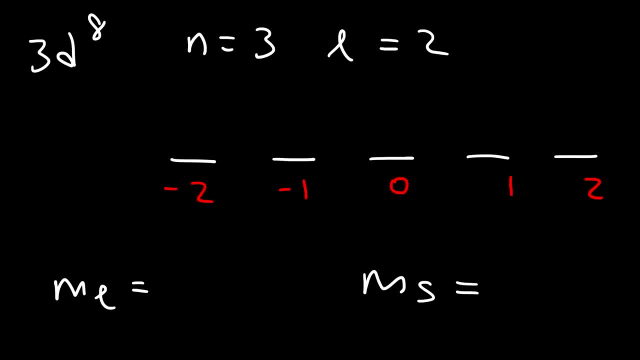 start with parallel spins facing upward. So this is 3d 1,, 3d 2,, 3d 3,, 3d 4,, 3d 5, 3d 6, 7, 8..